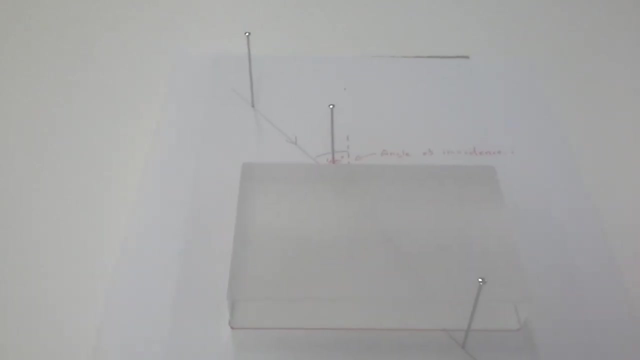 Hi guys, today I wanted to show you an experiment on how you can work out the refractive index of glass. I've got here a glass block and I've drawn around the glass block. Now this piece of paper is on a piece of cork board. 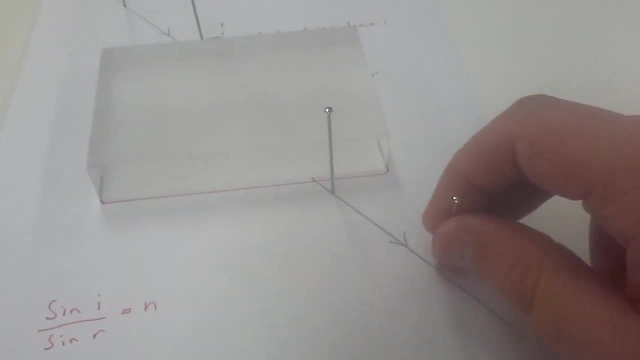 Okay, so there's the cork board there. I'm just going to take these pins out because we don't need them just yet, But I'll explain why the pins are there in a second. So first thing you do in this experiment is you place two pins into your board here. 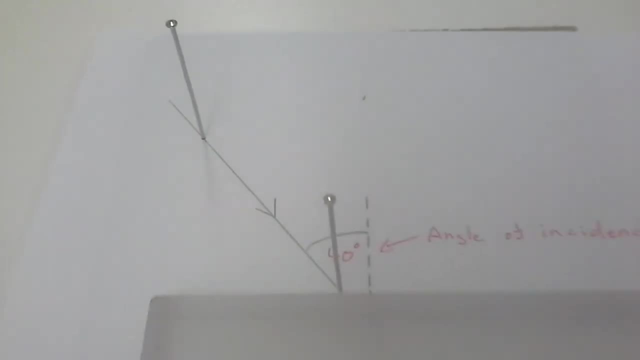 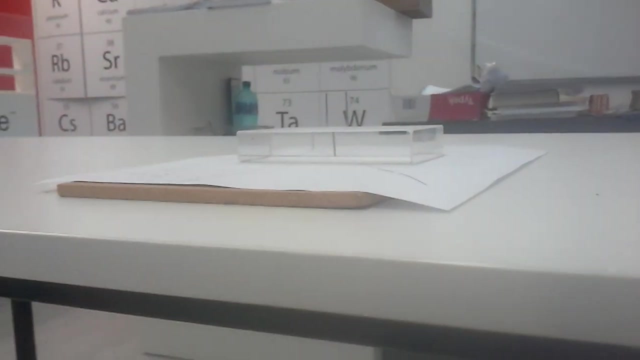 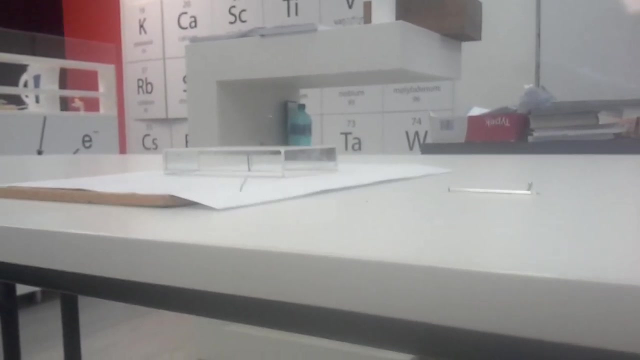 Just ignore the lines there for now. So you put two pins there and if I look like this at the refraction of the light coming from the pins, If I move it to the side here, if you look there, you can just see the image of the pins through the glass. 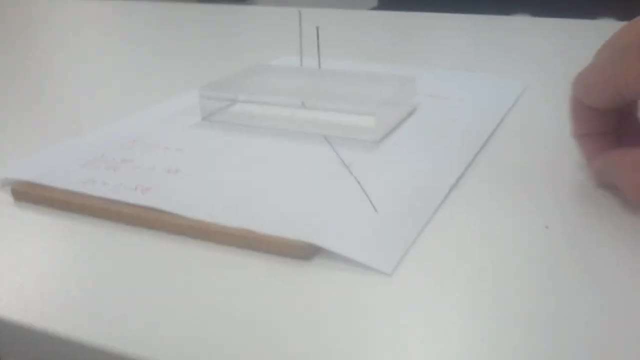 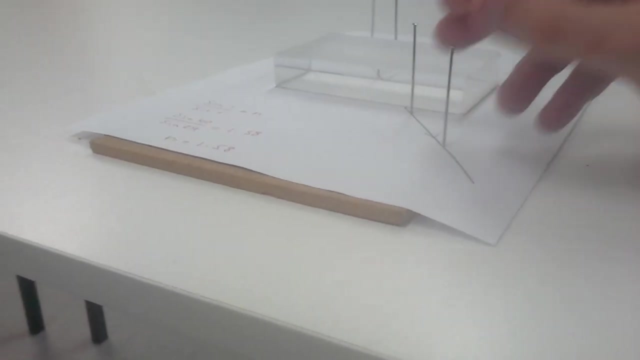 Now what I'm going to do is I'm going to get my pins here and I'm going to place them in line with the board With that image. Okay, like this. So if I'm looking through the glass, you can see the four pins there. 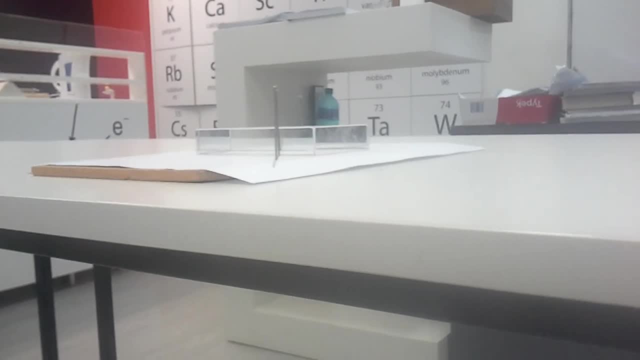 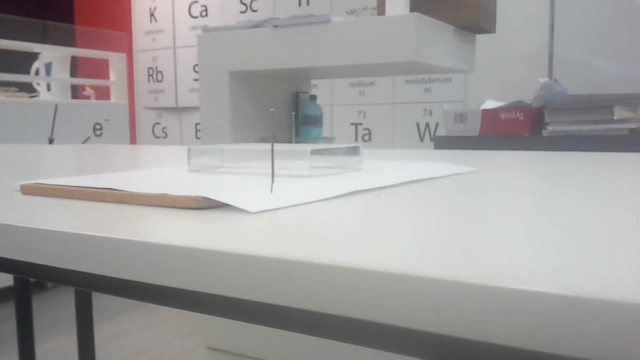 As I go, like this: you can see the pins. they all line up. Okay. so the image of the two pins and then the other two pins on this side. here You can see how they all line up. Okay, like that. 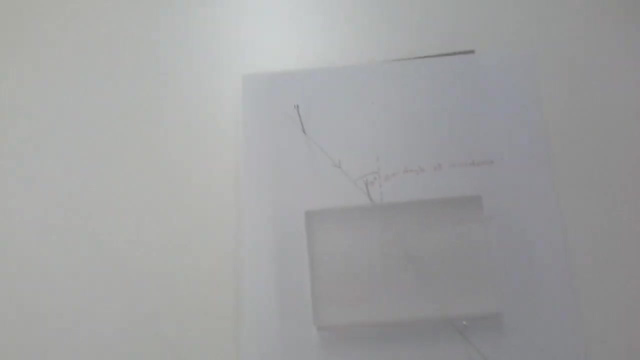 Then what you do is you remove the glass block- Okay, you've drawn around the glass block already. Remove your pins Where the pins have been. you can see two holes here. Okay, so you can draw a straight line there. 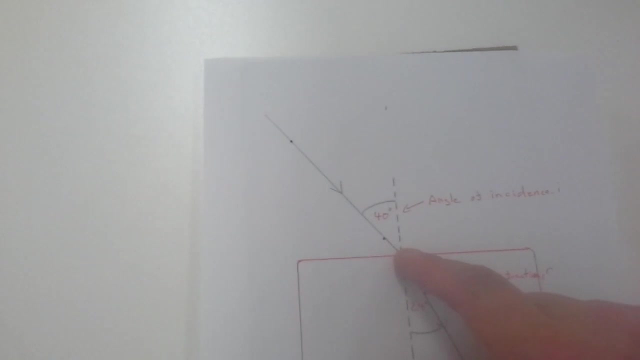 So this is representing the light going into the glass block. You need to mark the normal line there and then, using a protractor, measure this angle here, And this is what we call the angle of incidence and we're going to call it I. 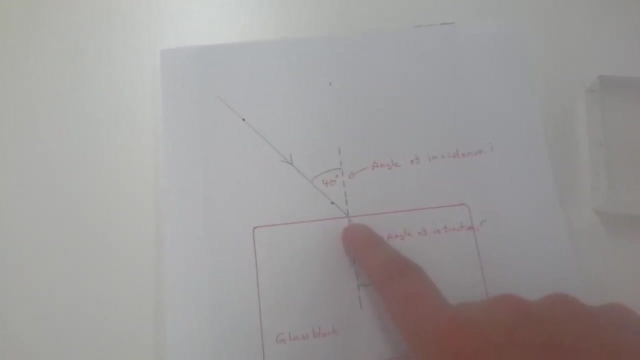 So in this case it was 40 degrees. Then you need to draw a line where this ray of light, this ray of light enters oops, where this ray of light enters here and then where it leaves here from the other two pins.